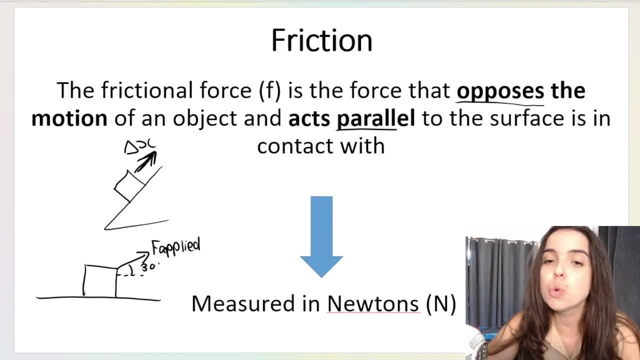 friction and the definition for friction is the frictional force, is the force that opposes the motion. and opposes the motion means acts in the opposite direction of the motion, So it contrasts the motion. So if someone is pulling a box to the right, frictional act to the left. If someone is 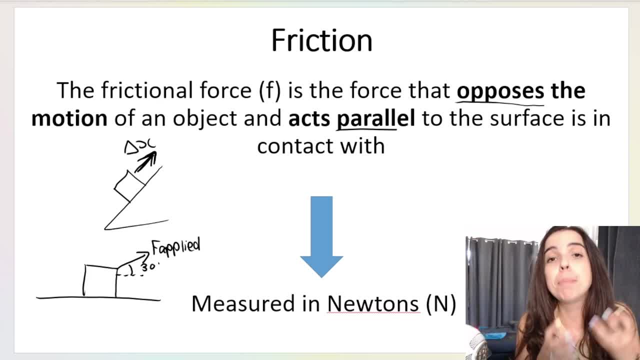 pushing or pulling a box to the left, frictional act to the right. So opposes the motion, goes opposite to the motion and acts parallel to the surface it is in contact with. So friction is a force exerted by a surface and it occurs when two objects are in contact on a surface. and because 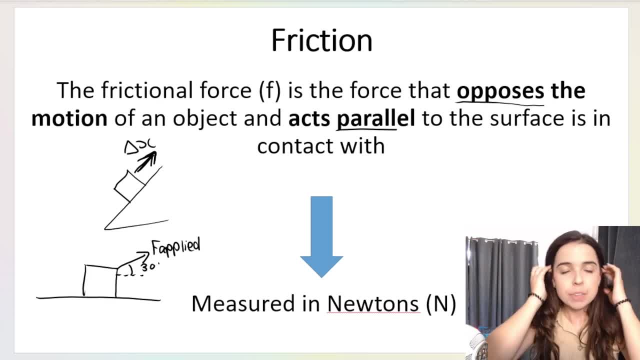 friction is a force. we know that the unit for friction is Newton. Now, very, very important if I have a situation where my object is on a horizontal surface over here and the object moves to the right, So the displacement of the object is to the right, or there's an applied force causing a. 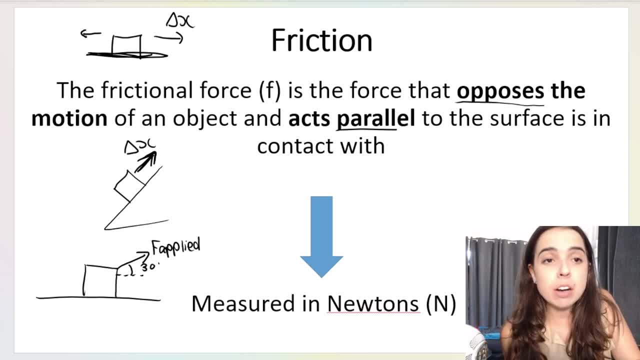 displacement to the right, friction will act to the left, parallel to the surface. So friction is always parallel to the surface. If I have an object being pulled up a slope, so you can see here, the displacement of the box is up the slope, friction will act down the slope. but it's important to note. 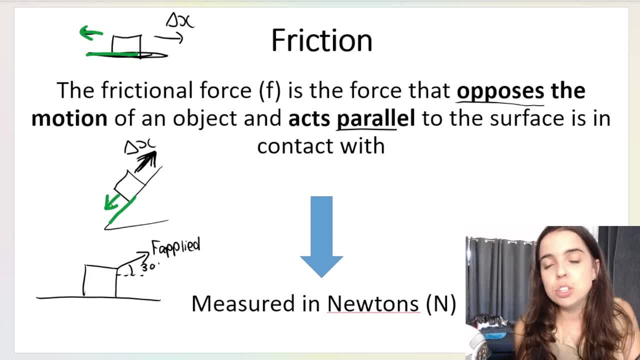 that friction is parallel to the surface and a lot of students get confused with this. If my box is pulled upwards at an angle of 30 degrees relative to the horizontal, So here you can see the supplied force is upwards at a 30 degree angle. Friction is not at an angle. Friction is always in the opposite. 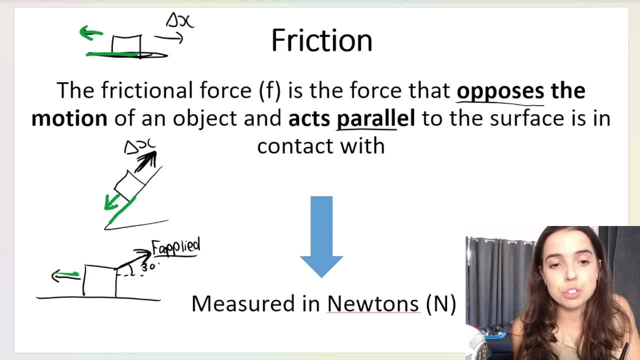 direction of the motion and it is parallel to the surface. So friction, once again, is parallel to the surface. That's the first very important thing to know about friction. The second is that we get two types of friction that we will be working with. So we've got static. 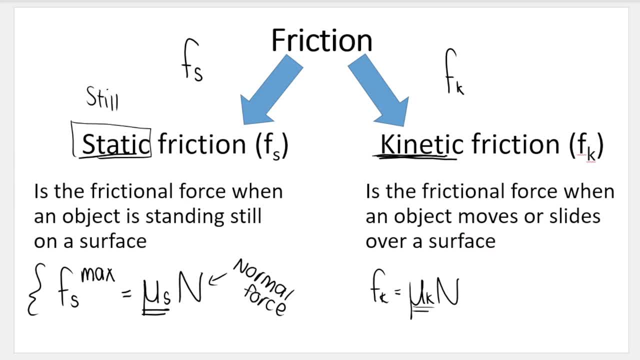 friction and kinetic friction. Now, as the name suggests, static friction is when we have an object standing still, So static friction is a frictional force when an object is standing still on a surface. There is an official definition that you need to know. it is in the exam guidelines, but this: 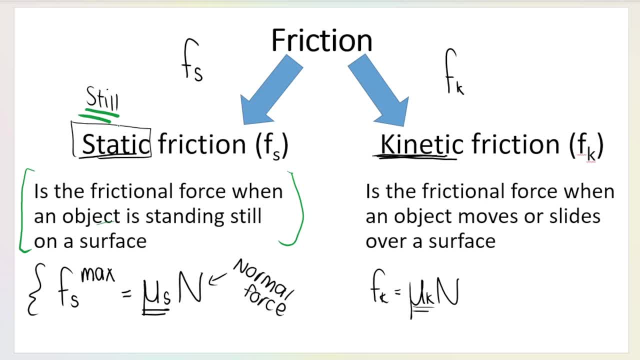 is just a very basic, brief definition in order to help you understand. And the symbol for static friction is F, So F like that, with a little baby S. Then kinetic friction. Kinetic means movement or motion, So kinetic friction is a frictional force when an object moves or slides over a surface. And these are the formulas that we're going to be. 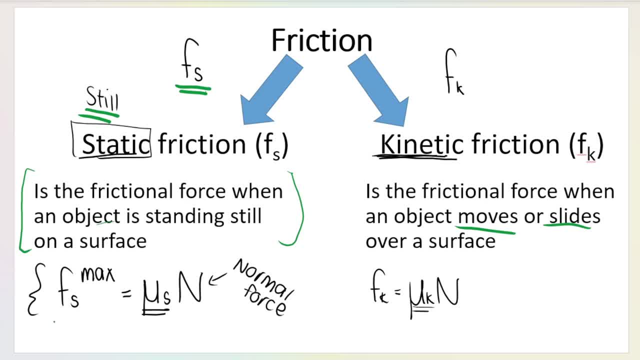 using to calculate friction. So maximum static friction. We take the coefficient of static friction multiplied by the normal force. I will explain what this thing means. This is called the coefficient of static friction. I'll explain what that means Very shortly, But for now just know that that's the formula, And for kinetic friction it's the same. 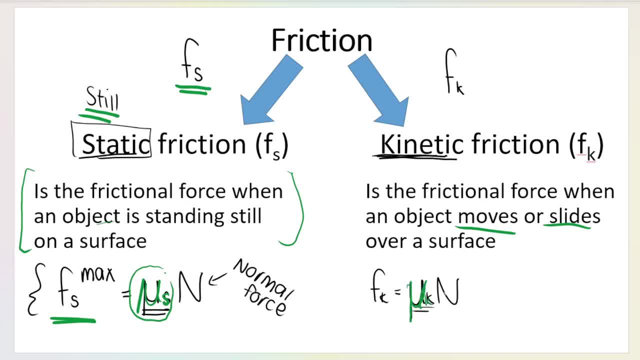 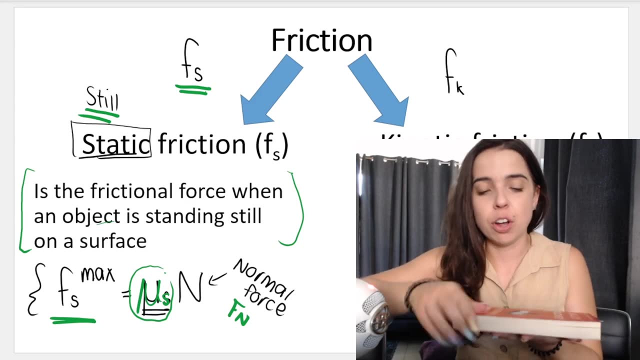 thing, almost, but it's the coefficient of kinetic friction multiplied by the normal force. Remember, the normal force is Fn or N. Right Now, there are technically three situations that you need to understand when it comes to friction, And they are as follows. Let's pretend that this is my surface. 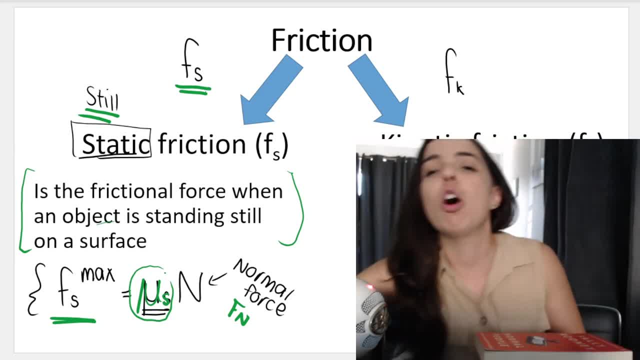 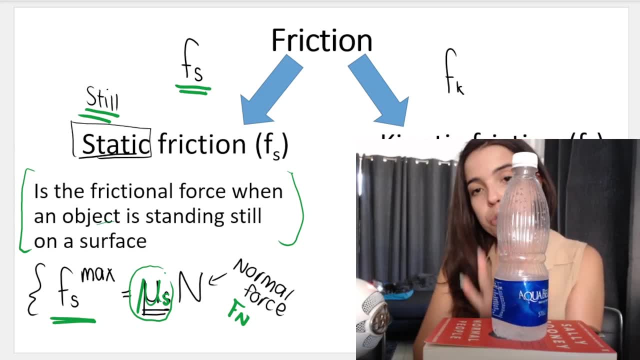 Okay, so here's my surface And here is my object. So I've got a water bottle standing on my surface. Do you agree that if you have to draw a freebody diagram for the situation, you'll have the weight of the bottle going down and the normal force of the surface acting upwards on the 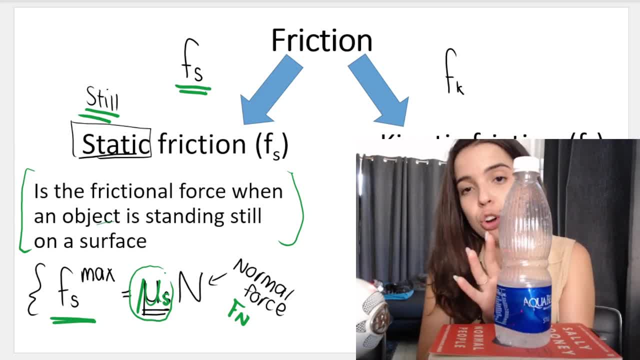 bottle. However, do you agree that there is no other external force applied on this bottle? In other words, I'm not pushing it, I'm not pulling it. No other forces are acting on this bottle. If this is the case, this object is going to be. 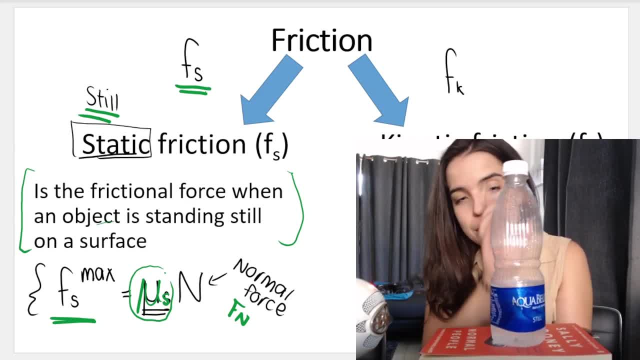 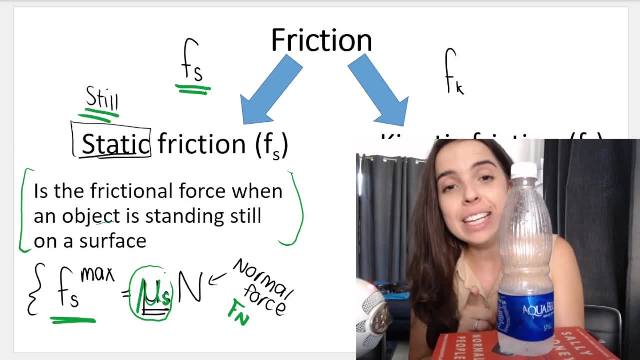 is standing still, but there's no applied force acting on the object. this object actually experiences no friction. no friction whatsoever, not even static friction. and you might say: but ma'am, didn't you just say that static friction is when the object is standing still? i did say that, but 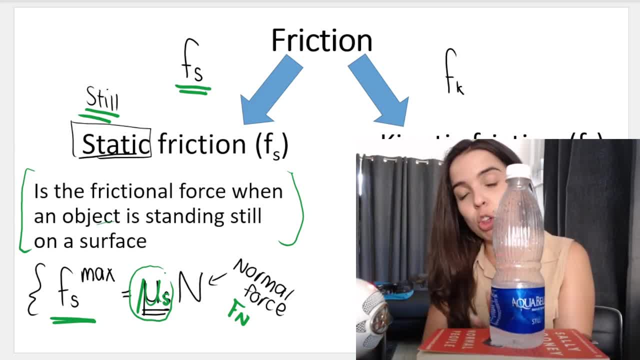 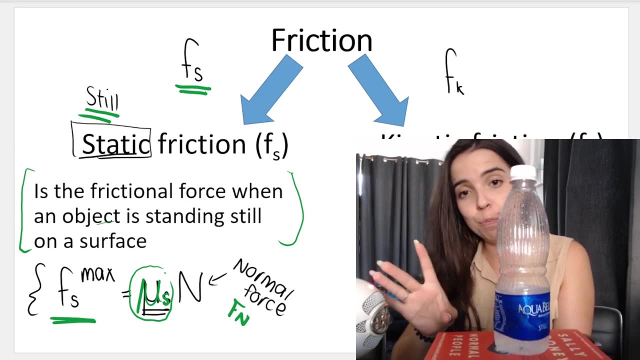 there's a difference between when the object is standing still completely and there are no external forces touching the object, and when the object is standing still but i have an applied force acting on the object and the object is still not moving. so look at the difference: no external force applied at all. object is standing still, no friction as soon as i apply. 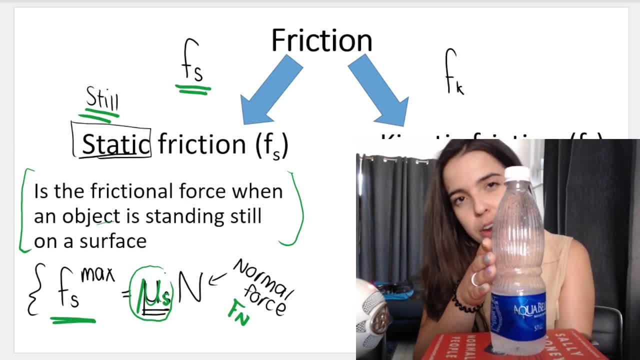 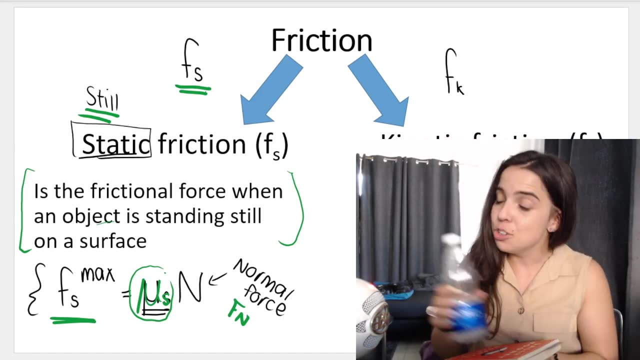 force. now take note how i am applying a force. it's a very, very small force. is the bottle moving? no, however, i am applying a force. i'm applying a very, very, very slight force to the right, okay, but the box, the bottle, is not moving. in that situation, 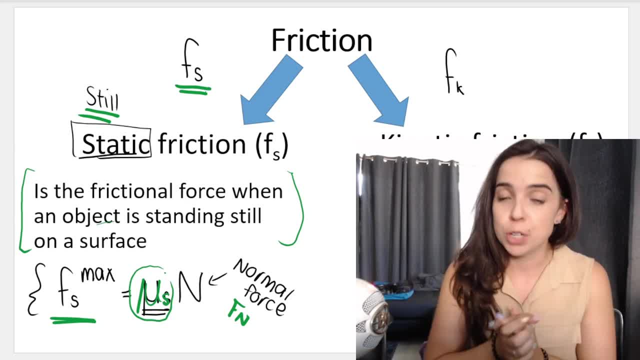 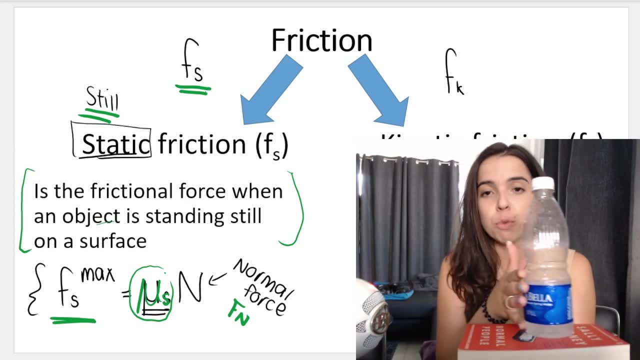 when there is an applied force acting on the object and the object doesn't move, that's when we have static friction and then obviously kinetic friction will be. when i'm applying the force and the object moves, then there will be kinetic friction. so i hope you understand the 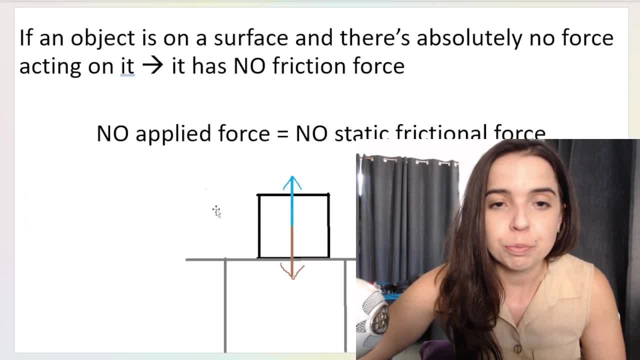 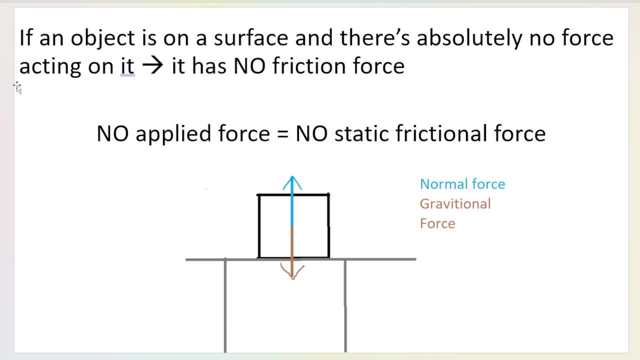 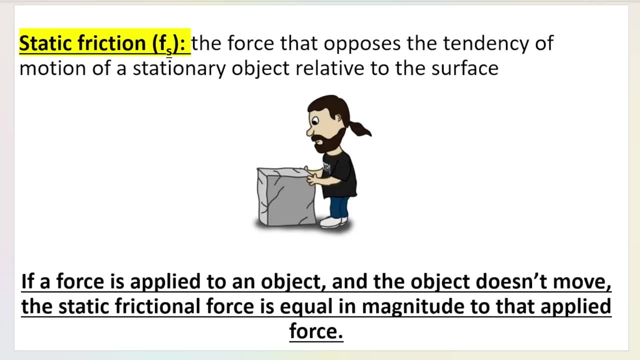 difference. so if we take a look at this note over here, it says that if an object is standing still on a surface and there's absolutely no force acting on it, it has no friction force, no applied force, no static friction, no friction whatsoever. however, as soon as i apply a force to the object and the object does, 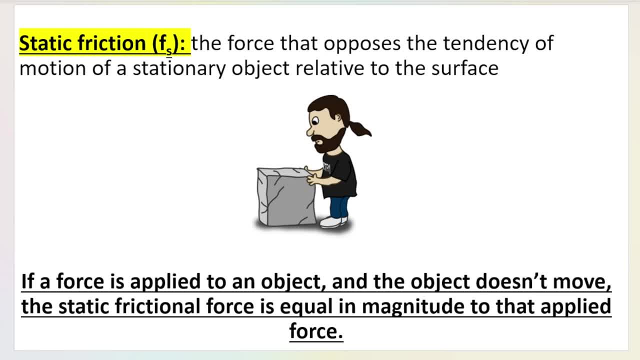 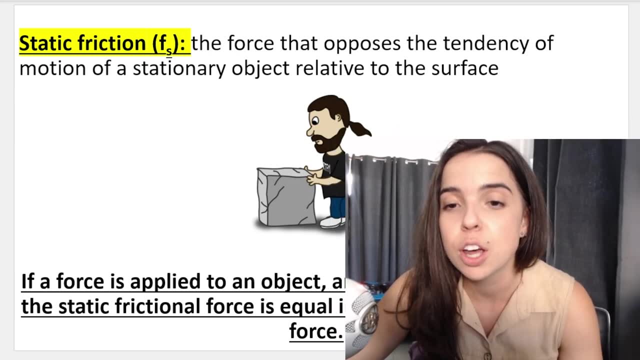 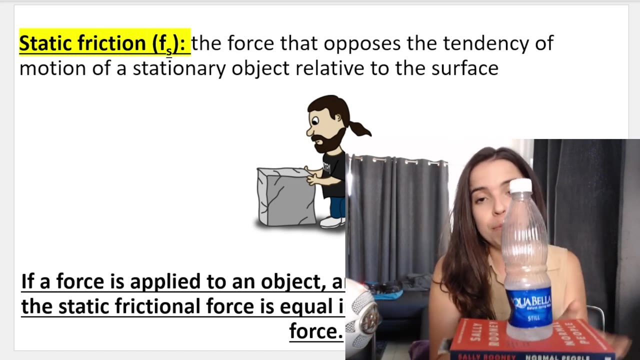 not move. there's static friction, and that static friction is equal in magnitude to the applied force. here's the proper definition for static friction: the force that opposes the tendency of motion of a stationary object relative to the surface. so it applies. it opposes the tendency of motion of a stationary object. so, in this scenario, absolutely no applied force. therefore, we have no. 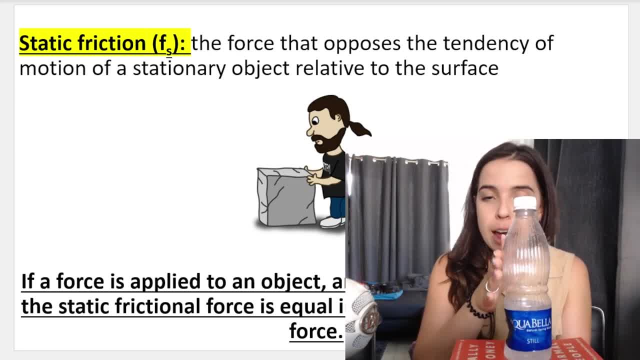 static friction. but as soon as i start to do this, i have an applied force on this bottle, but is the bottle moving? no, so therefore the bottle has static friction. if i apply a force of one newton to the right, static friction is one newton to the left. if i increase the force, i'm pushing a little bit. 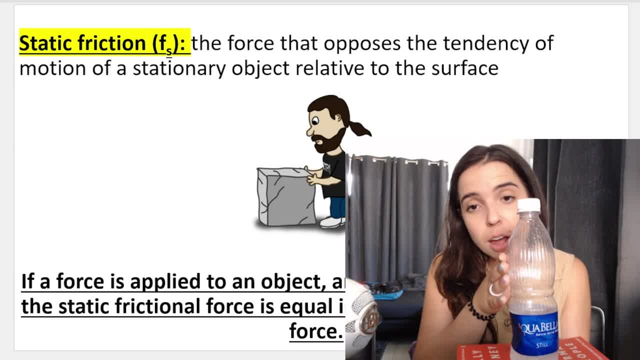 and i'm pushing with two newton to the right, applied force of two newtons to the right bottle still not moving. so static friction is two newtons to the left. I continue pushing a little bit harder, a little bit harder, a little. 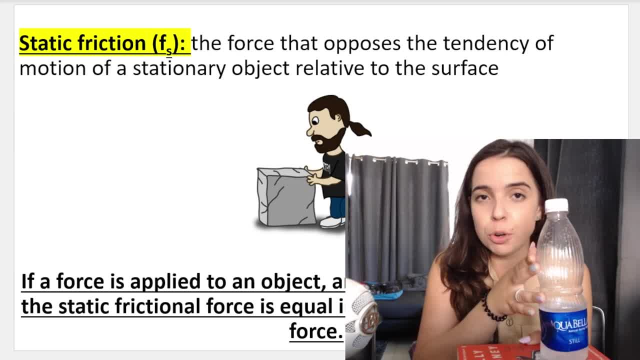 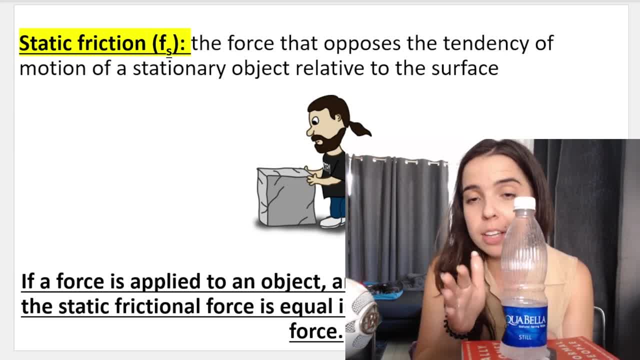 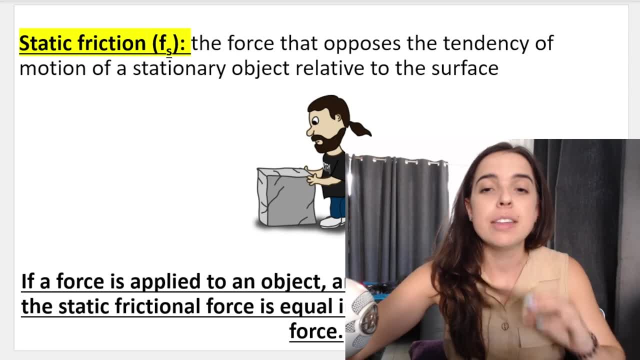 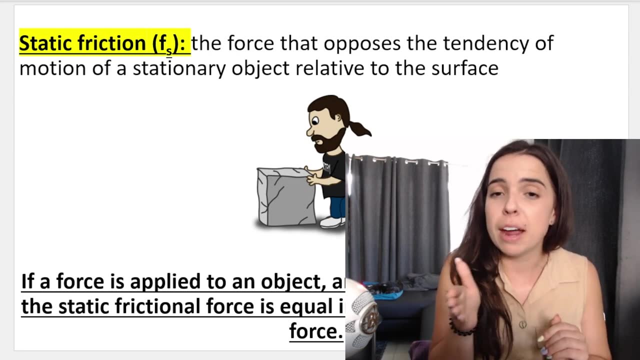 I push it harder, harder, harder, until it eventually is on that point, that tipping point of moving, That point, just, just, just as it starts moving, we say that it has a maximum static friction. and if I push harder, if I apply, if I have exert an applied force just more than 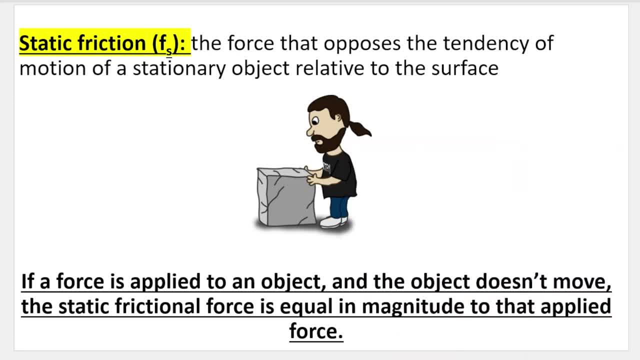 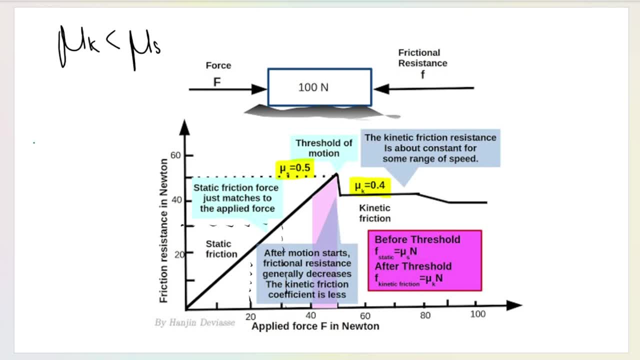 that, then it'll start moving. Okay, then it has kinetic friction, and the way that I can represent that is in a graph like this. So, as you can see here at the bottom of the graph, remember I said: if I have, let's say, 10 newton of applied force, let's first read our 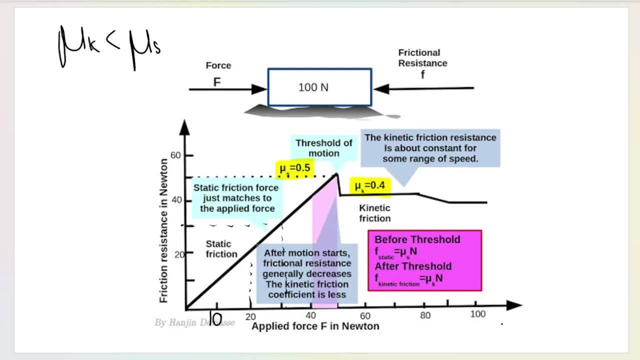 axes. it's very important when you look at graphs to read your axes. the x-axis has applied force in newton, so that's how hard I push the applied force. and then the y-axis has frictional resistance in newtons, in other words friction Now in the beginning, if I apply a force of 10 newton. 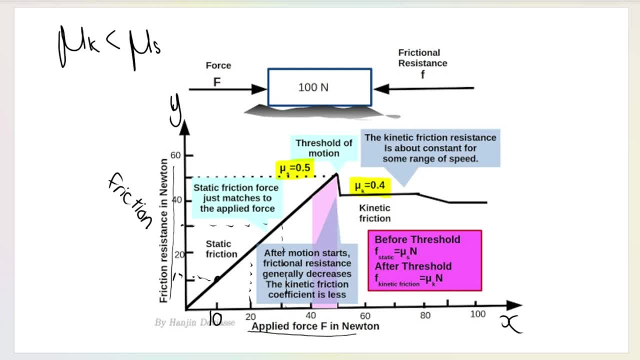 the object's not moving. static friction is 10 newton. I increase my applied force to 20 newton. the object is still not moving. static friction is 20 newton. So basically, what's happening is this: I'm pushing to the right with 20 newton. that is my applied. 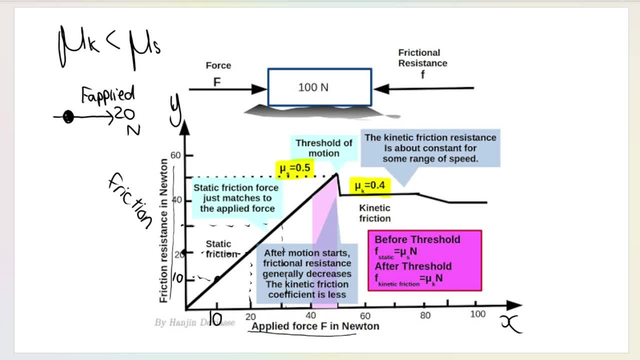 force or f applied and because the object is not moving. static friction is also 20 newton, but in the opposite direction. Remember positive 20 minus 20, that gives me f net of 0. That's why the box is not moving. 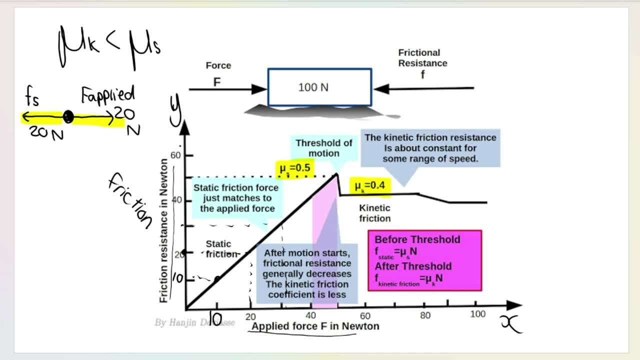 okay, it's stationary. we continue increasing our applied force: 30 newton applied force, 30 newton static friction. 40 newton applied force: 40 newton static friction. so we have a straight graph until it reaches this point over here, and that point over there is what we call f s max. it's the 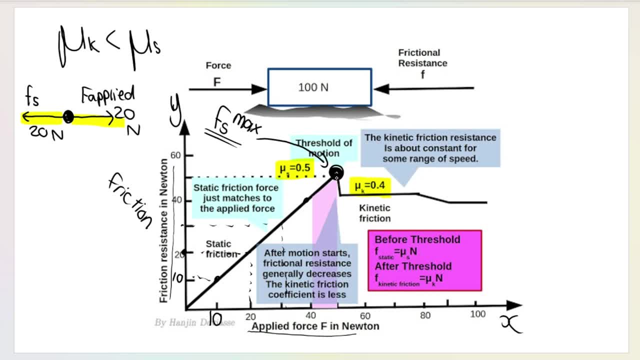 maximum static friction. when my applied force goes beyond that point, then my object starts to move and you can see that friction drops. kinetic friction is constant, more or less so it says your kinetic friction is about constant. we don't say about constant, we take it as constant for the 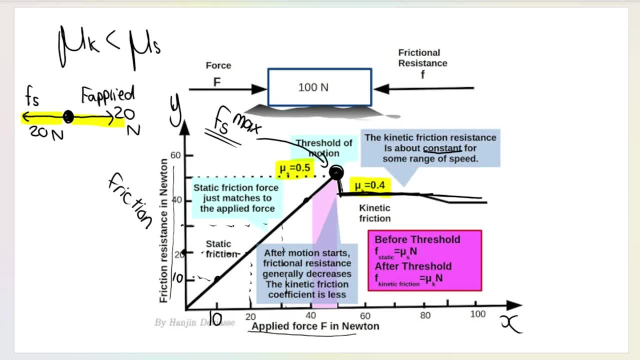 same range of speed. okay, and one thing that is interesting is that there is a drop, and that is because kinetic friction is always less than static friction. one of the reasons is because the coefficient of kinetic friction- so that is the symbol- always smaller than the coefficient of static friction, and that's what i wrote over there. 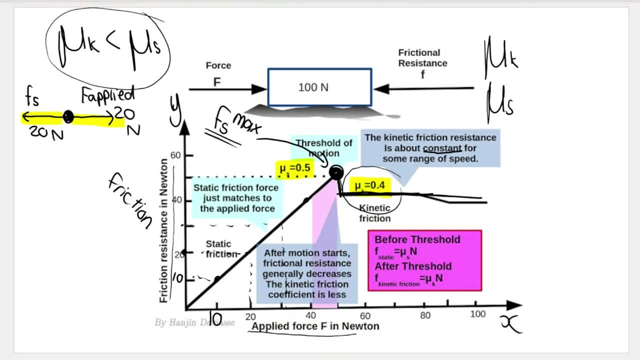 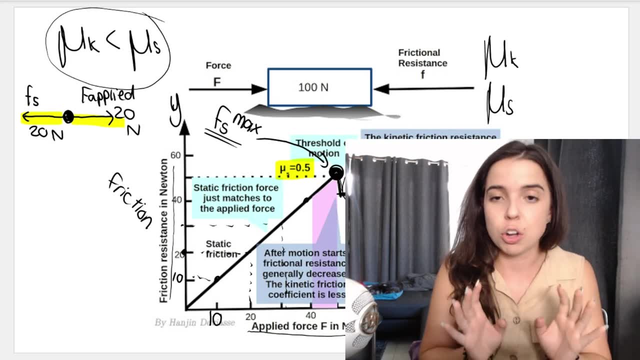 and another way to think about this that makes sense is if i'm trying to push a very, very heavy box- very, very heavy- think about the heaviest box you've ever pushed across a carpet takes a lot of efforts to get it to start moving. remember you must increase your applied force, increase your 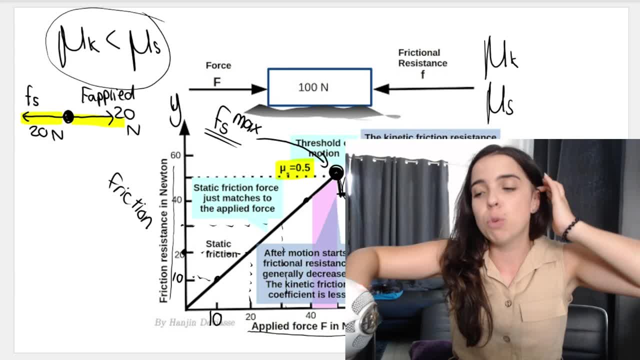 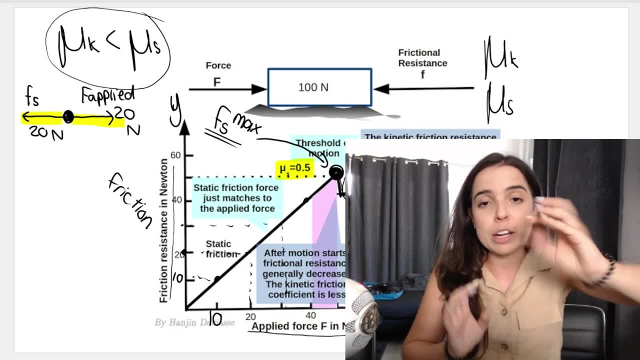 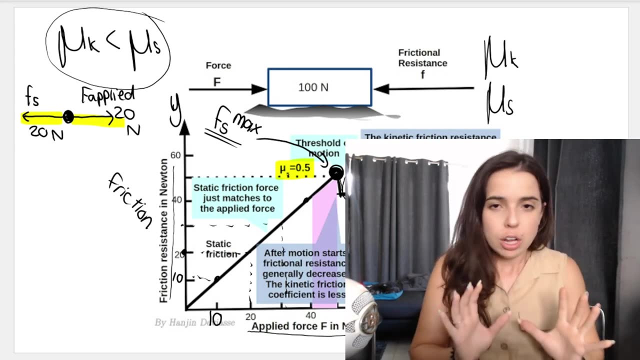 applied force. increase your applied force, keep increasing your applied force until you reach that fs max. so you're pushing very, very, very hard, increasing, increasing. you reach fs max, you push past that and then the box starts to move. is it more difficult to get the box moving or to keep it moving? okay, so it's more difficult if you. 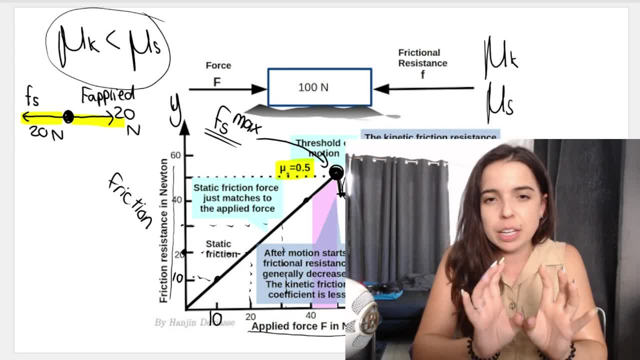 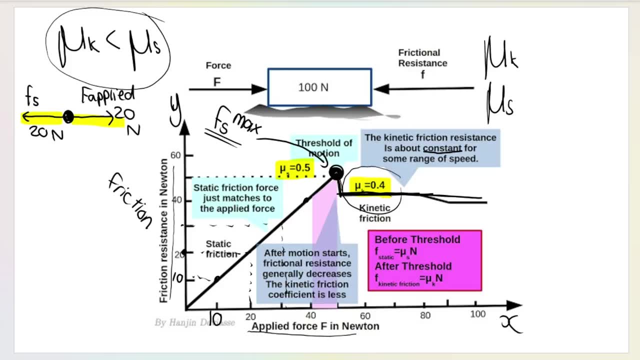 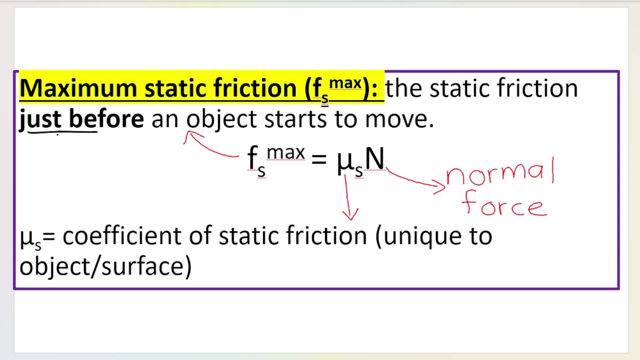 think about it to get the box to start moving. once it's moving, we can keep it going. it's easier. so kinetic friction is less than static friction. okay, now, as i mentioned, this is the formula to calculate maximum static friction. so it's a static friction just before an object starts to move. 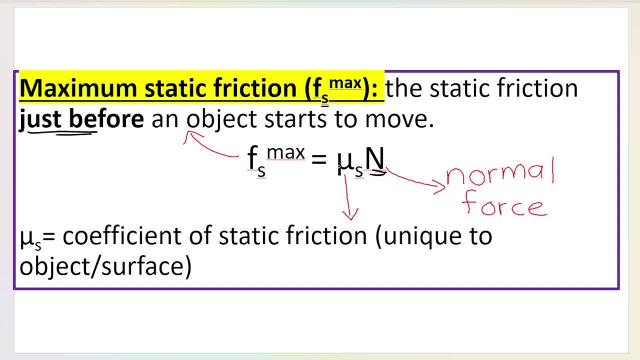 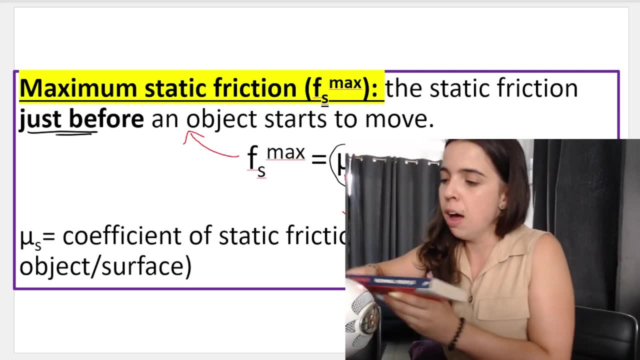 remember i told you that n is the normal force. this is the coefficient of static friction, and i wrote here that it is unique to objects or surfaces. now what that means is that that coefficient, if i have my bottle and this book, they have their own unique coefficient of static. 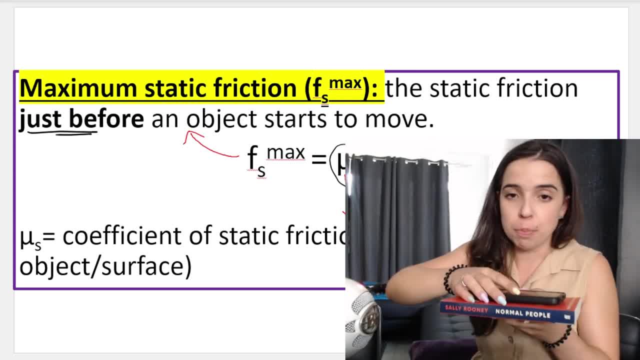 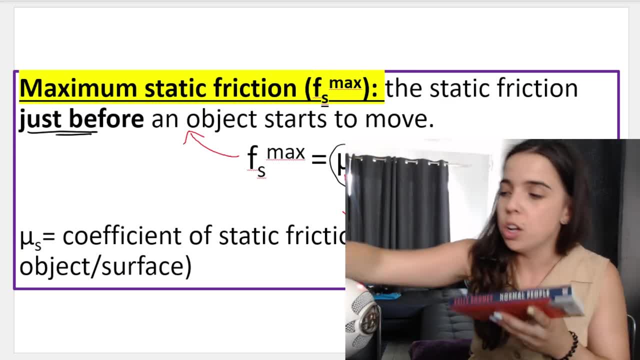 friction if i have my cell phone and this book- two different objects, so remember it was bottle and book- it has static friction. so if i have my cell phone and this book- two different objects, so has its own coefficient- phone and book- it has its own coefficient of static friction. so every set of 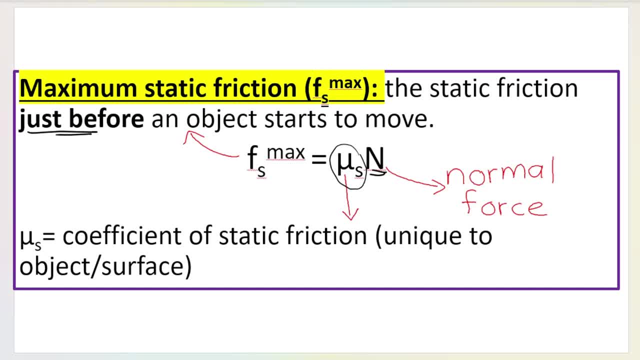 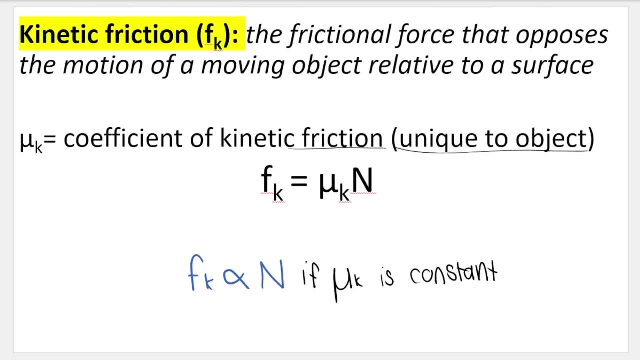 objects has their own coefficient of kinetic friction that is unique to those two objects, and this is how we calculate kinetic friction. and the one thing that i do want you to pay attention to with these formulae is the following relationship that i wrote out for you here: 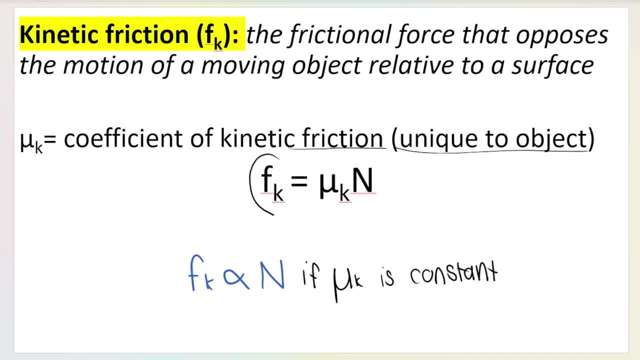 the frictional force is directly proportional to the normal force if the coefficient is constant, which it is constant if we use the same two objects. so this little funny symbol over here, that means directly proportional. and what that means is if the normal force increases, the frictional force increases by the same proportion. so if i double normal force, frictional force, 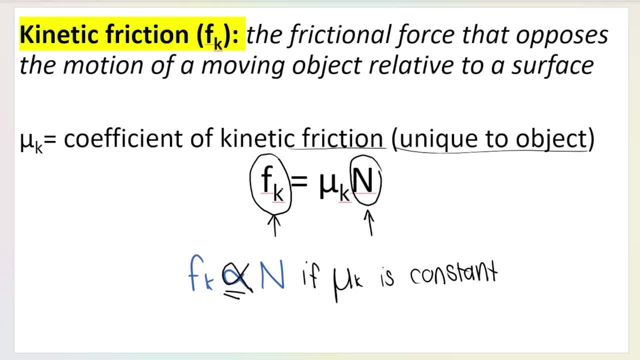 will double. If I halve the normal force, frictional force will halve. So basically, if n goes up, friction goes up by the same proportion. If n goes down, friction goes down by the same proportion. And if that doesn't make sense to you, you can always just prove it to. 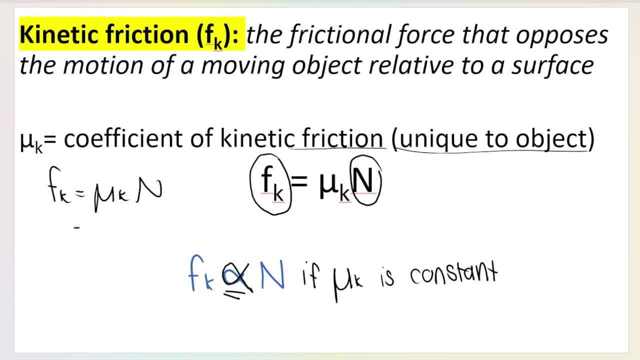 yourself quickly. Let's pretend my coefficients of kinetic friction is one. It's usually less than one, but let's say it's one. And let's say my normal force is initially two Newton. What is one times two? Well, we get two. Now if I keep my coefficient the same. so I'm keeping it one. 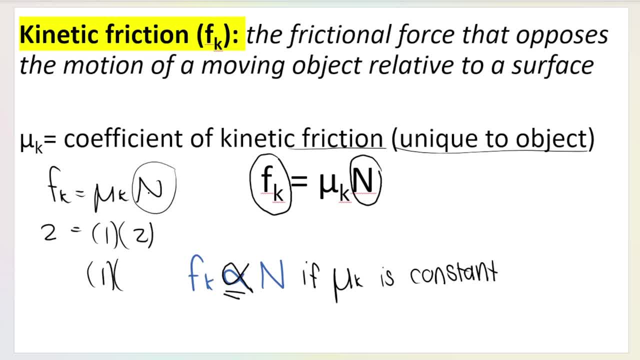 and I triple my normal force, So two. how do you triple it? Times three, So that is six. Then one times six is six, So this also triples. That relationship will always be true if the coefficient is constant. That is very, very important to understand Now. 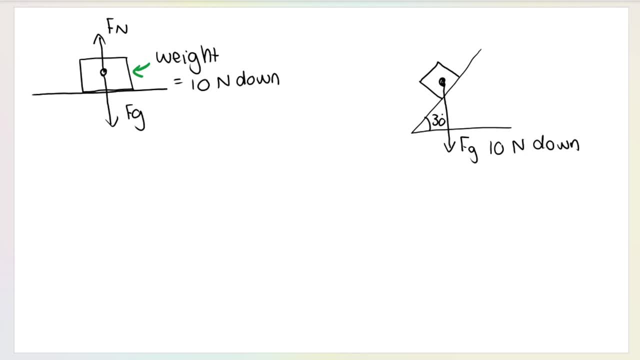 when we get to the point where we're going to get to the point where we're going to get to, we need to consider the weight. the weight and therefore the normal force, Because, remember, to calculate kinetic friction, we need the coefficient which depends on the surfaces. 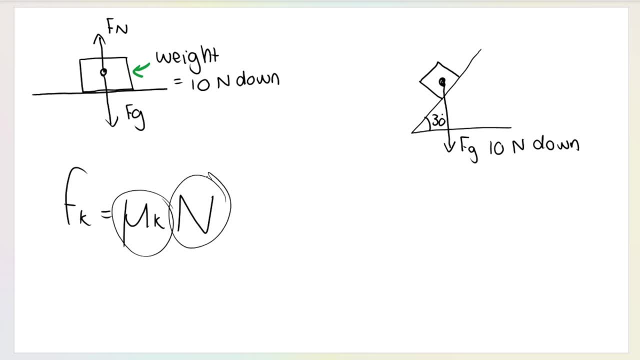 and the normal force. Normal force we often get by using or considering the vertical forces. So I did this in the previous video, but you will recall that in this scenario over here I only have the normal force acting up and Fg acting down. The normal force and Fg together give me zero. 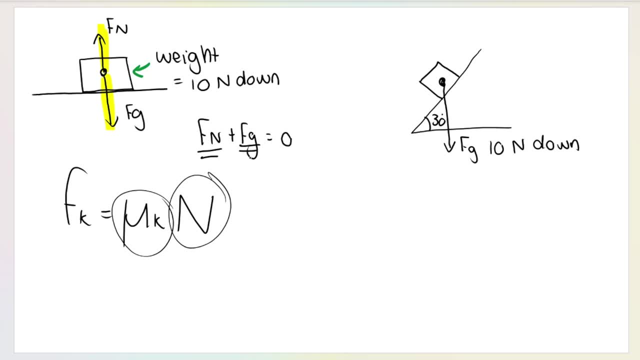 which means that the normal force and the weight force are equal in magnitude but opposite in direction. In this situation over here, where the box is on a slope, remember, the normal force is 90 degrees to the surface, or perpendicular to the surface, like that. That's Fn And we can also. 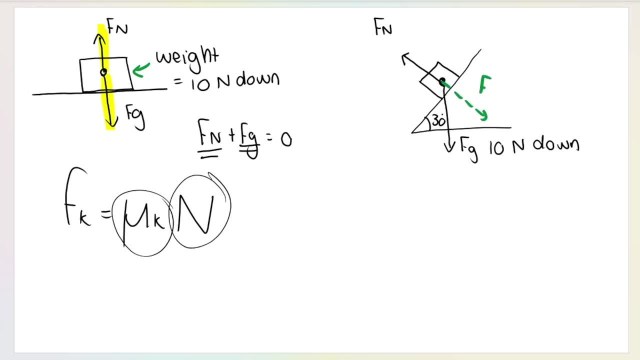 resolve weight into its components like this: That's Fg perpendicular and this is Fg parallel. And if you watched the normal force, you will know that the normal force and Fg perpendicular- those two are equal in magnitude. Now again, why do I care about this? Because I need to use this information to help me work. 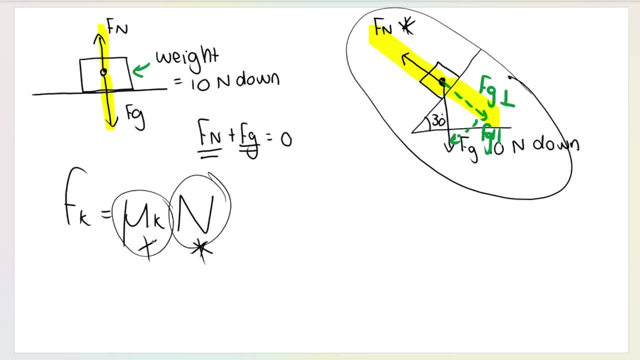 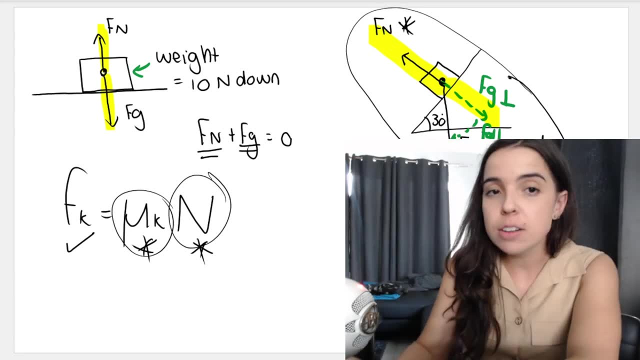 out the normal force And once I have the normal force and I have the coefficient, I can work out friction. So if you missed the videos that I did where I worked out weight, the components of weight, and then we moved on to the normal force and how to work out the normal. 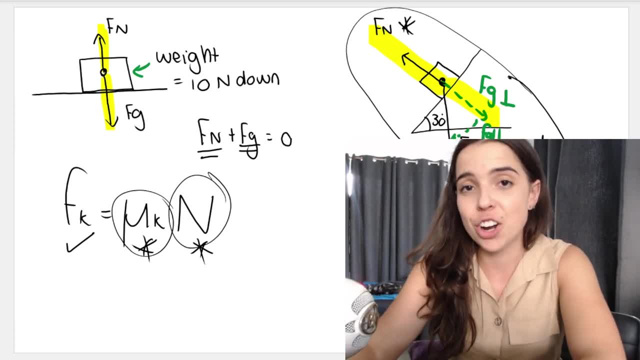 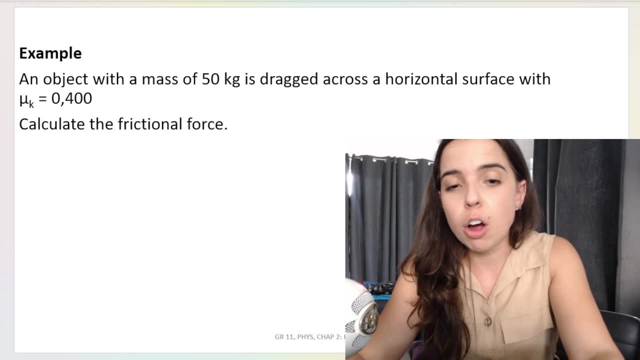 force for different situations. please, please, please, check out that video. I will link it in the description box below. You need to know that in order to be able to tackle friction. But before we move on, let's do this calculation for friction. 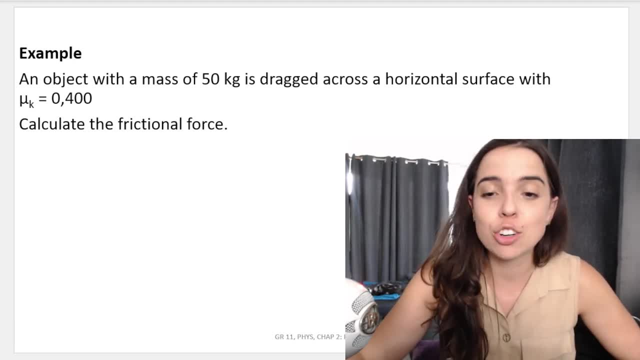 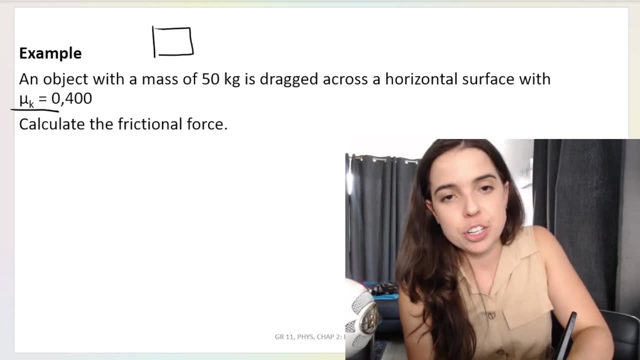 So it says an object with mass 50 kilograms is dragged across a horizontal surface and they give you the coefficient of kinetic friction. So basically we have a situation like this: we have a surface and we have the object being dragged or pulled. let's assume to the right by a F applied. 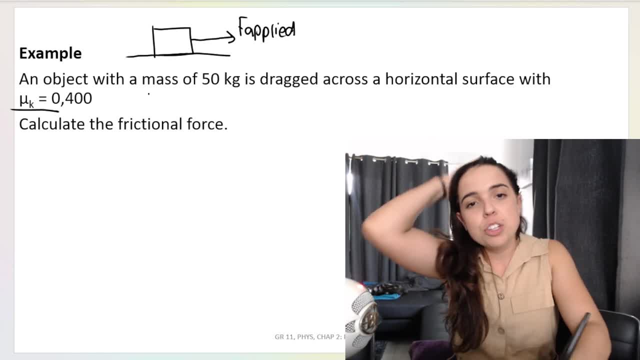 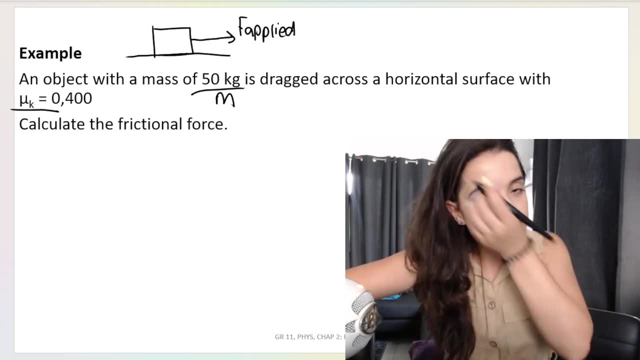 we have a surface and we have the object being dragged across a rough, rough horizontal surface. they give me the mass, which is important. I do need that, that's M, and they give me the coefficient of kinetic friction and they want the frictional force. Now how I recommend starting this question. 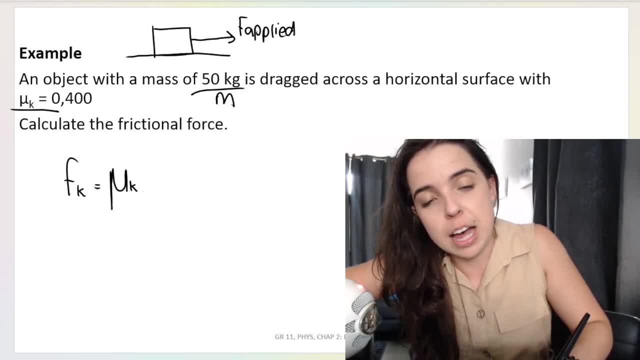 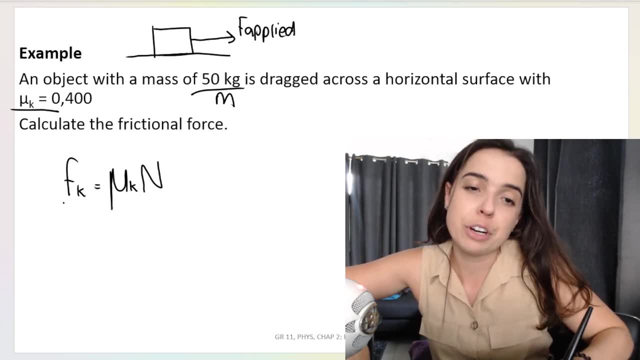 is with the formula. FK equals the coefficient of kinetic friction times n. Now if you look at that, you should see the following: I want the frictional force, So that's where my question mark is going to go. I want the coefficient of kinetic friction. But in order to use this formula, I first need to work out. 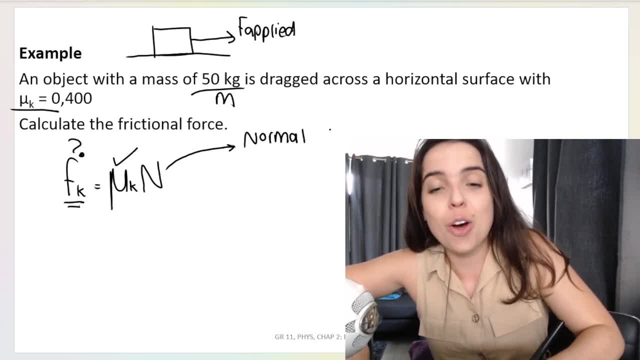 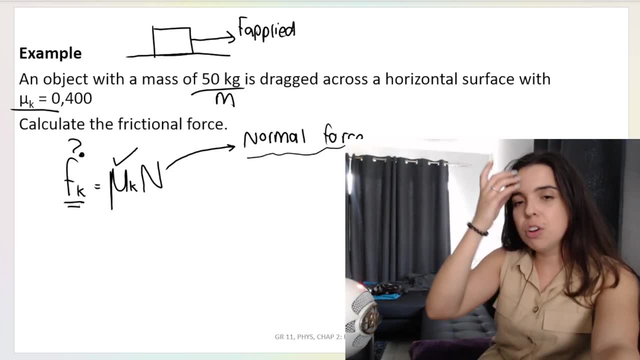 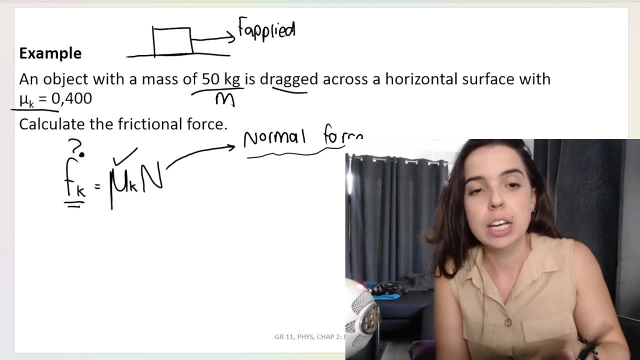 the normal force. So this is why it is important to know how to work out the normal force. So I hope you've watched that video And my students also often ask me about. how do you know that you must use FK and not FS? Well, because the object is being dragged, So there is motion and they give. 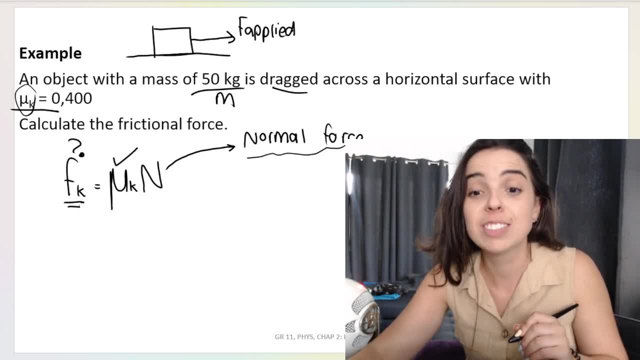 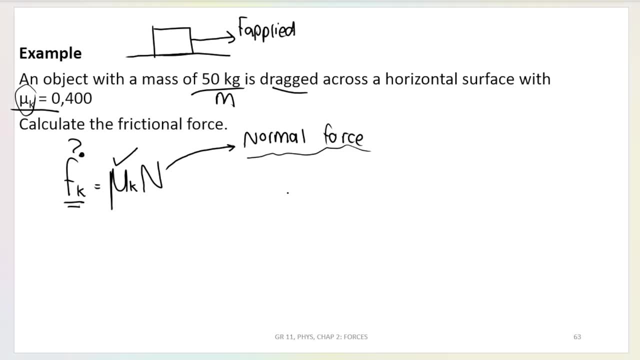 me the coefficient of kinetic friction, which means we need to work out kinetic friction. Okay, how do I do this? How do I work out the normal force? Well, remember, if I draw a free body diagram to help me with the scenario, I have FN acting straight up, I have FG acting straight down, I have the applied force acting to the. 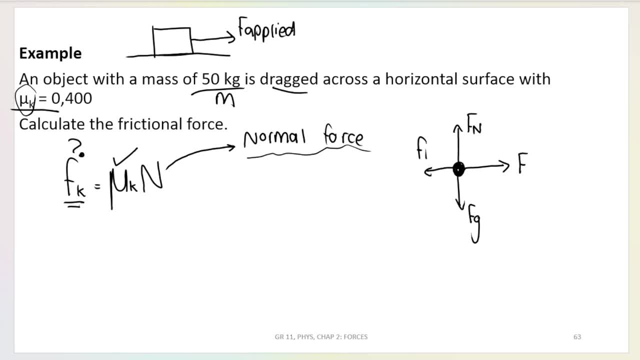 right, I'm just going to call it F and I have FK, or the friction, acting to the left. How do we do this? What do we do? Well, we first need the normal force. Now take a look at where the normal force is. It's over here, And because it is, 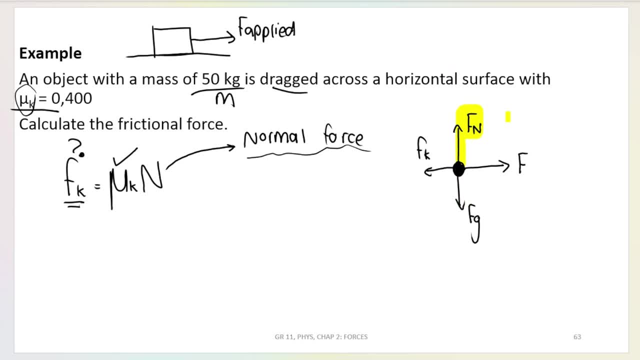 acting 90 degrees. we need to work out the normal force. So I'm going to work out the normal force. So I'm going to work out the normal force. Now I'm going to take the force and it's going to be square, which is going to be the force, which will be acting 90 degrees to the surface. So it's in this y direction, or this perpendicular direction, or this up. 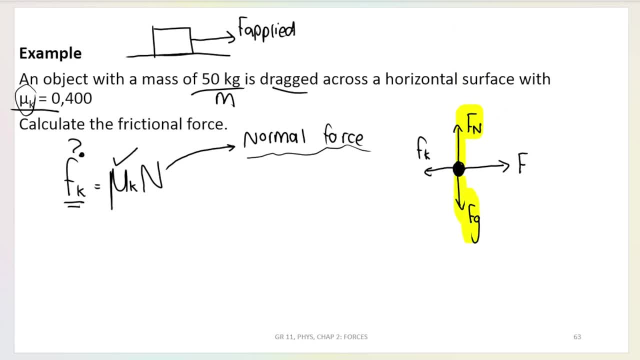 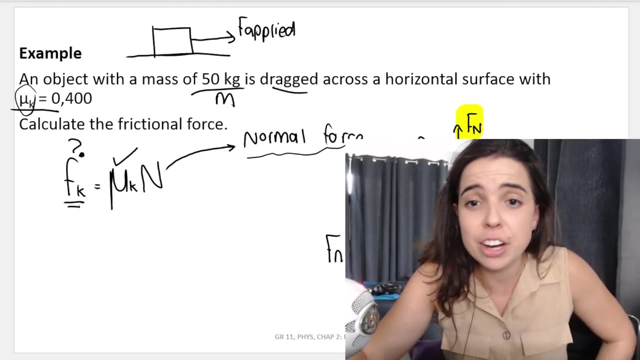 down direction. I'm going to consider all the forces in that direction. So I hope you remember from the previous video that we go F net in the y direction must be zero. Now, this often confuses learners and they say: but ma'am, why must F net in the y direction be zero? Because, remember, think about the box. the box is sitting on a surface. 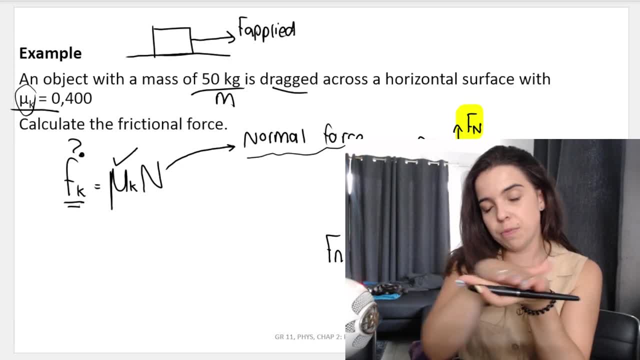 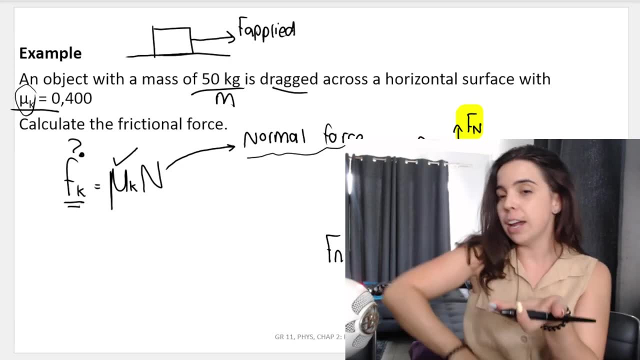 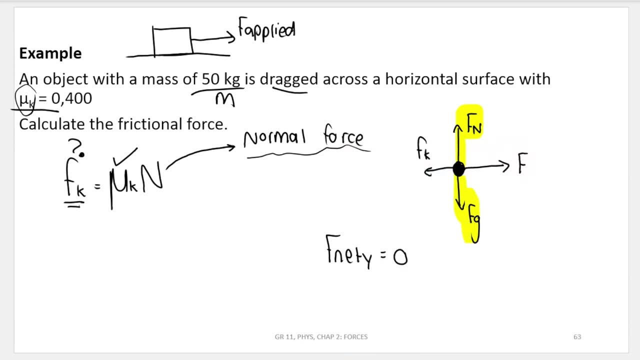 even though the box is being dragged in the this direction. so we're dragging the box to the right, the box is not moving in this direction. think about it. the box isn't going or like flying down. it's moving this way. so that means the forces in this direction- the vertical direction- is zero. now, which forces do i care about? because i am: 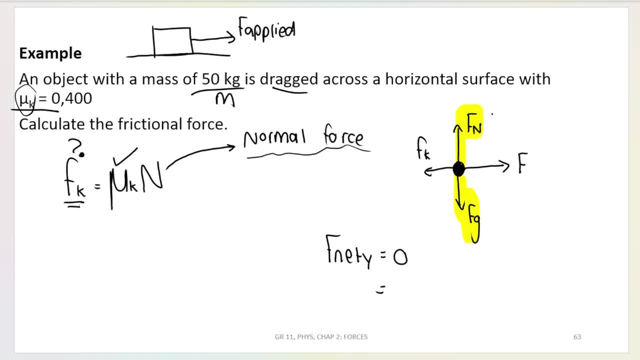 looking for f n, this one. i care about f n and f g because both of them are acting in the y direction, the up down direction. i make it equal to zero, i'm choosing up, like this is positive and f n is what i'm looking for. because f g goes down, i'm making it negative. now, how do you calculate f g, remember? 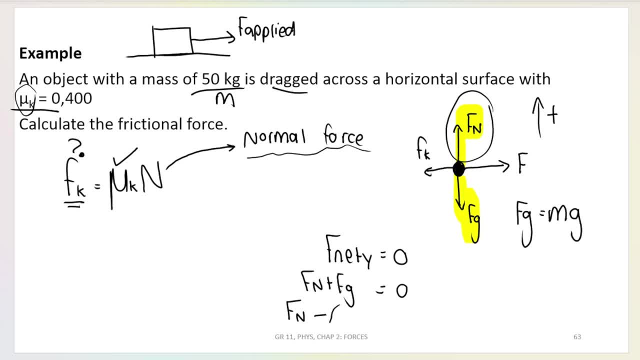 f, g is equal to mass times gravitational acceleration. so it's your mass, which is 50 times your gravitational acceleration, which is 9.8. that gives me zero. you take over the 50 times 9.8 and it becomes positive 50 times 9.8.